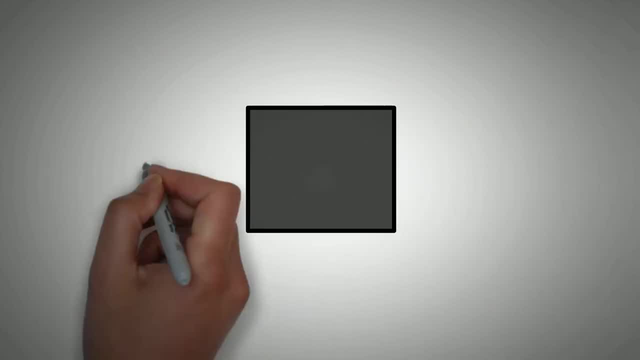 think of a cryptographic hashing algorithm like a magical black box, where you give it something and then it poops something out. A hashing function is just a system where you can put something into it and it'll output a hash. So we'll get into what a hash is in a second. 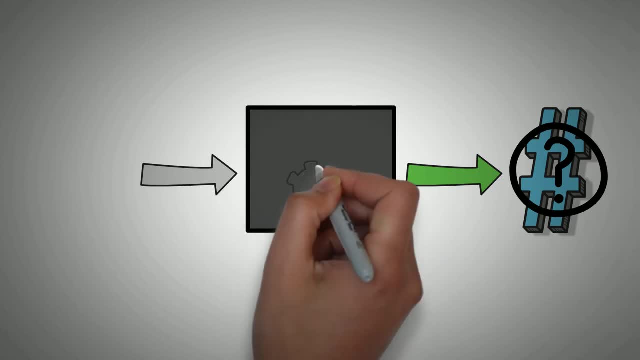 but just know that we do need it. Now there's a ton of math happening inside this so-called magical black box, but essentially you give it something and then it does the pooping. In this case, Bitcoin uses the SHA-256 hashing function. Now there's many different types of 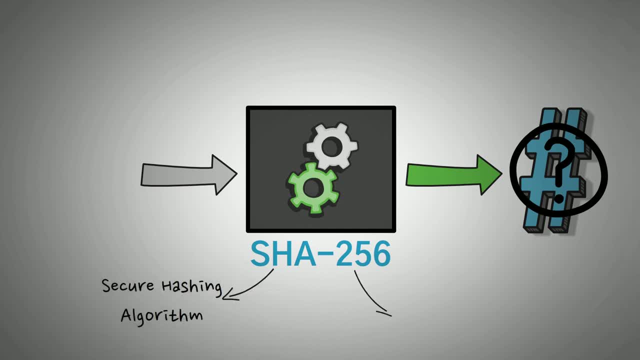 functions, but SHA stands for Secure Hashing Algorithm, and 256, refers to the amount of zeros and ones that it has in whatever it outputs. So whether you put in your name or you put in the entire dictionary, what it poops out will always be 256 ones, and 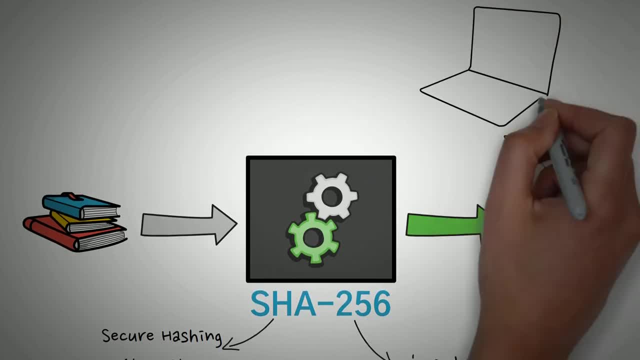 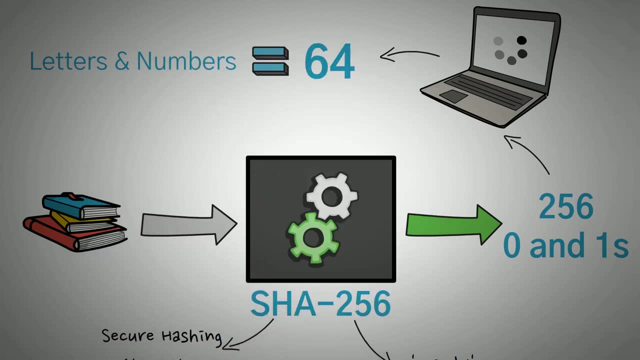 zeros. Now our computers are really smart, so they convert these ones and zeros the binary- to actual letters and numbers, which equals 64 numbers and letters. Now, there's many different hashing functions, but Bitcoin uses SHA-256, and in this video we're going to focus on that. 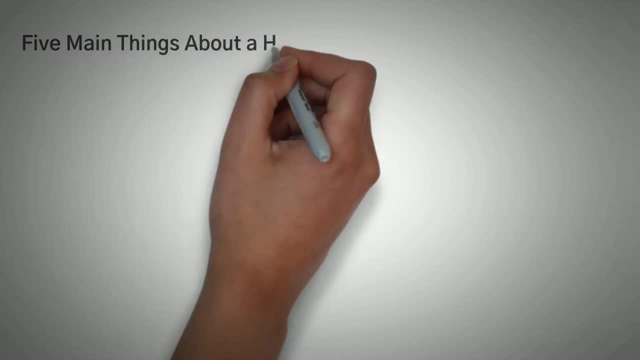 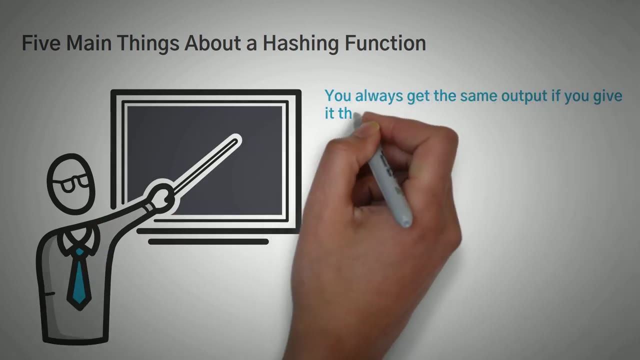 function for examples, So let's get into it. Essentially, you need to know five main things about a hashing function. Number one: you always get the same output if you give it the same input. Number two: no matter how much data you give it, it always poops out the same size of output Number. 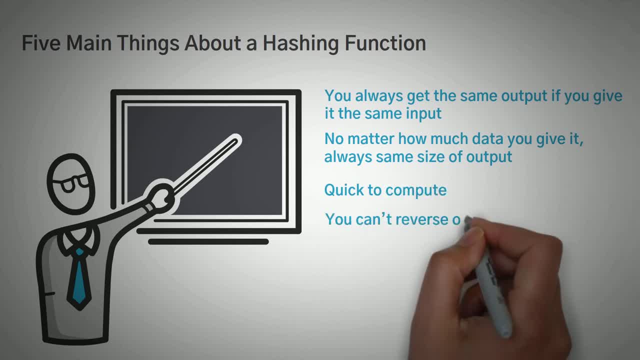 three: it is quick to compute. Number four: you can't reverse it or predict the hash. And number five: it's infeasible to find two hashes with the same input. So let's go back over these in a little bit more detail. Number one: you always get the same output if you give it the same input. So if 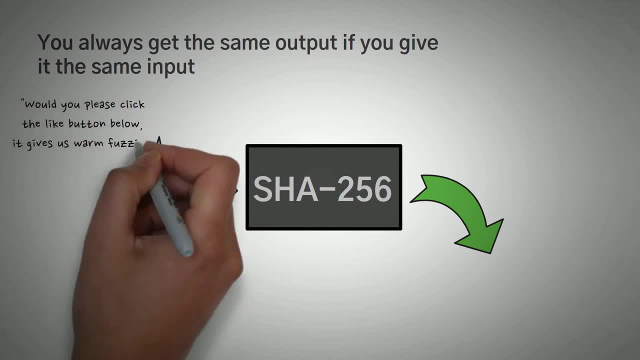 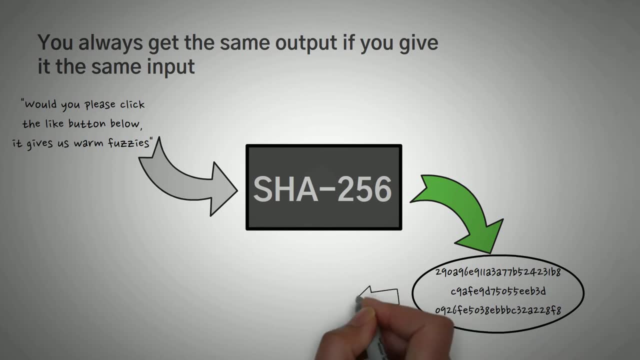 we give it. would you please click the like button below? It gives us warm fuzzies. Then it would output this: But if you did it again, it would give you the same, seemingly random numbers and letters, but they will be the exact same. Now, these numbers and letters are what? 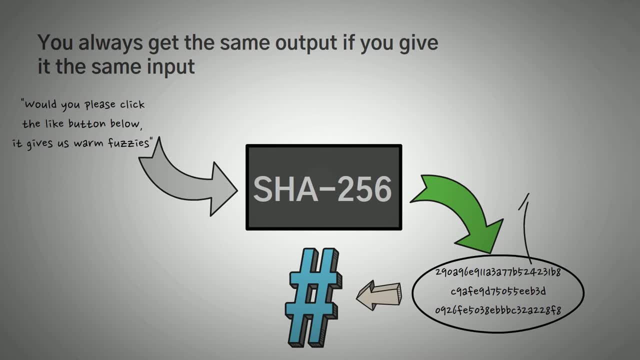 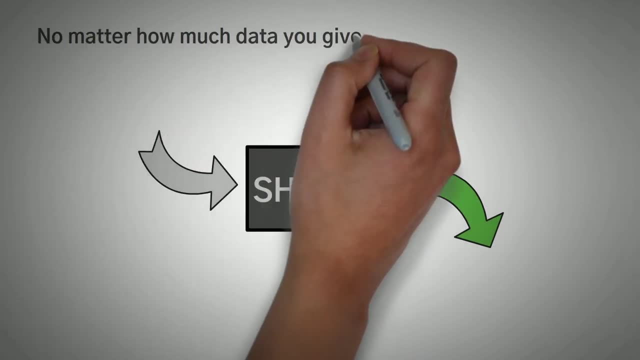 we call the hash And, like I said, it's actually a bunch of ones and zeros, but we turn it in the number and letters so we can look at it easier and it's easier to copy and paste. Number two: no matter how much data you give it, it'll always give you a fixed output. So if you give it an A, 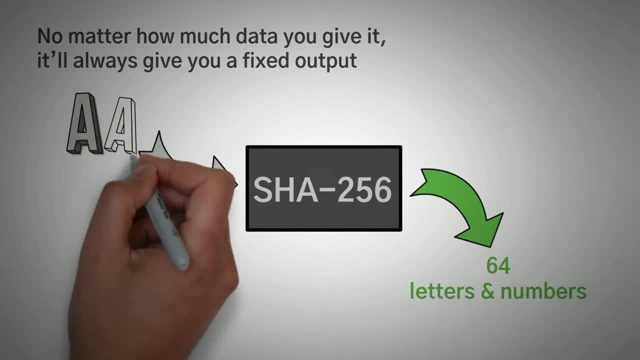 it'll give you 64 numbers and letters. If you give it AA, it'll give you 64 numbers and letters. Then, if you give it AAA, it'll give you 64 numbers and letters. Then, if you give it AAA, it'll give you 64 numbers and letters. And if you give it the entire encyclopedia. 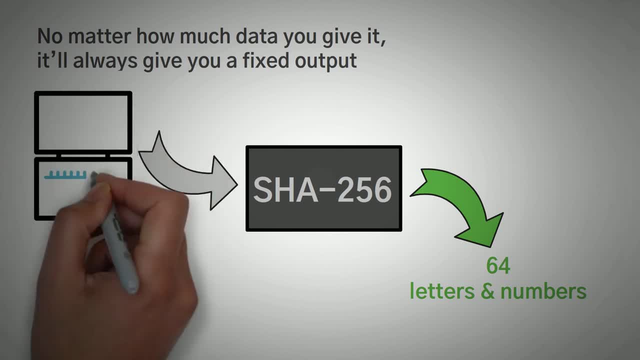 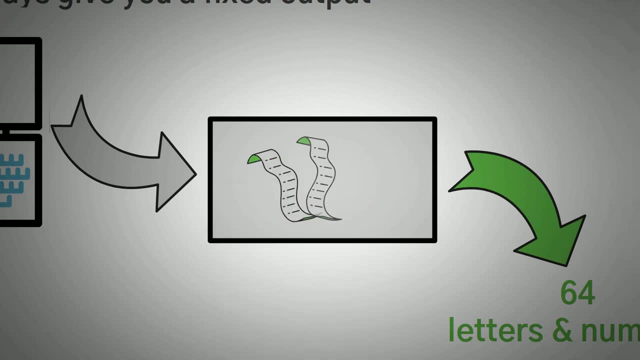 it'll give you 64 numbers and letters. And lastly, if you gave it my social security number, it'll still give you 64 numbers and letters. The black box is magical in this sense that if you give it a letter or a million letters, it'll always output 64 numbers and letters. Number three: 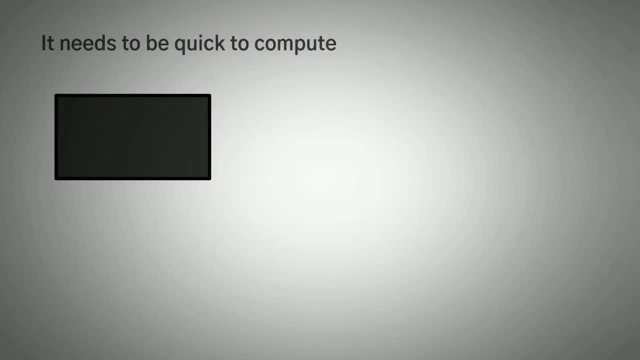 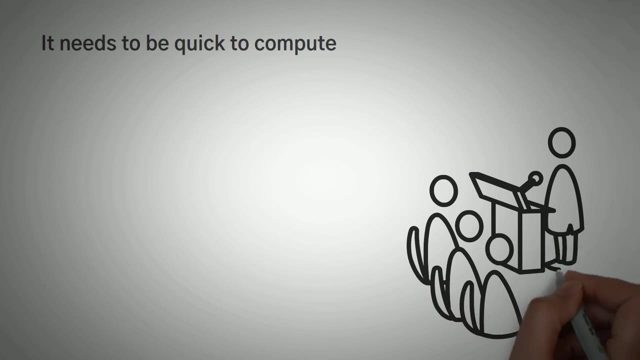 it needs to be quick to compute, So this would be a really good place to show you exactly what's going on inside this hashing black box, but it's very technical and not everyone who watches this video really needs to understand completely how it works. If you do. 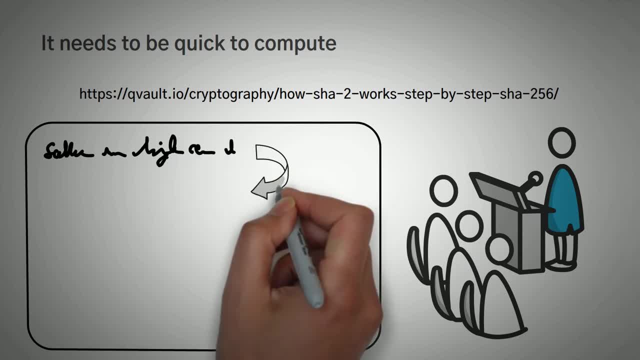 though. here's an intro. See, it first converts your message to binary, and then it adds a single one, and then it adds zeros until it gets to a multiple of 512 ones and zeros. Then it appends 64 bits, then it initializes hash values, and this is where most people will have to look up. 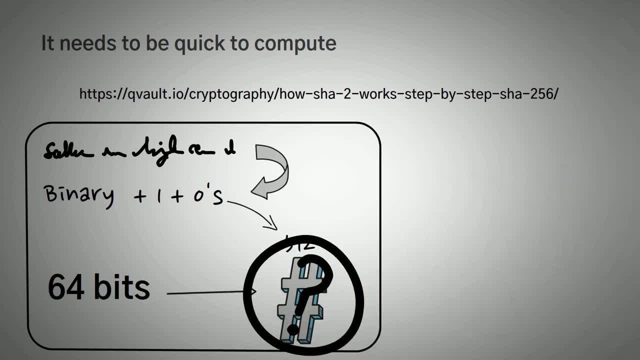 what initializing hash value means, And that's why I'm not going to explain the whole thing, because just look, message schedule, chunk loop. you don't need to know exactly how all these work. to know how a basic hash function works, You just need to know that it basically does a bunch of 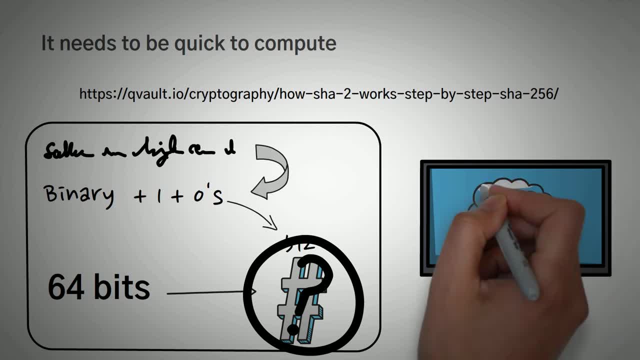 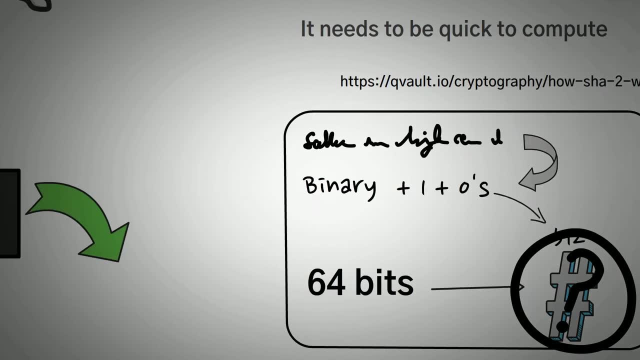 math with the ones and zeros. Computers are really good at math. so that sums up our third point, that it needs to be quick to compute, And actually most computers can do a few million of these each. second Number four: changing the input, just a. 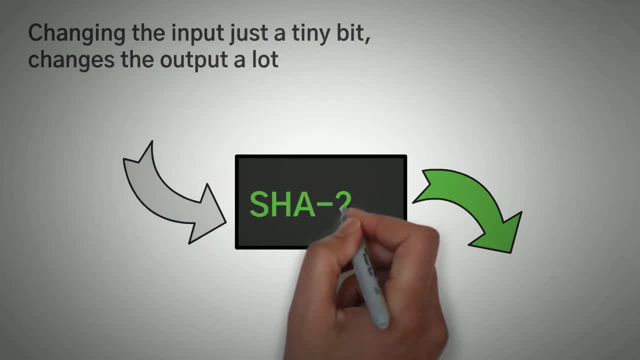 tiny bit changes the output a lot. So, basically, if you do SHA-256 of subscribe to our channel, you get this as the output. However, if you do please subscribe to our channel, you get this, which is entirely different. And lastly, if you change it just a tiny bit, we're just going to 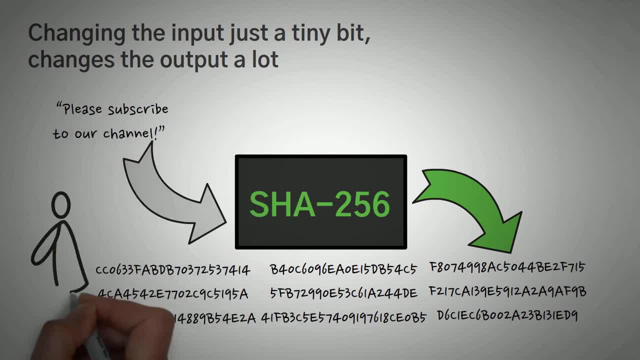 add an exclamation point. You get this as the output And there is a reason. we want a small change in the message to graph out the output. So if you do this, you get this as the output, change the hash because otherwise it might be predictable And that would break the security. 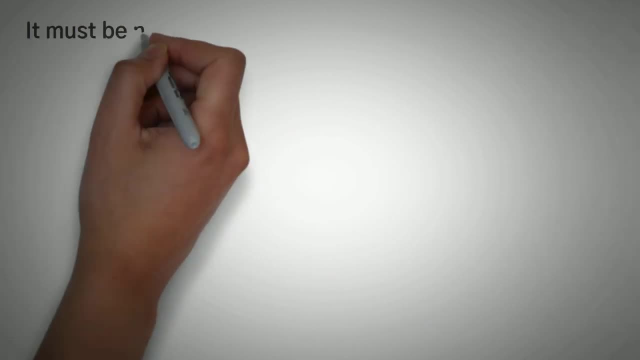 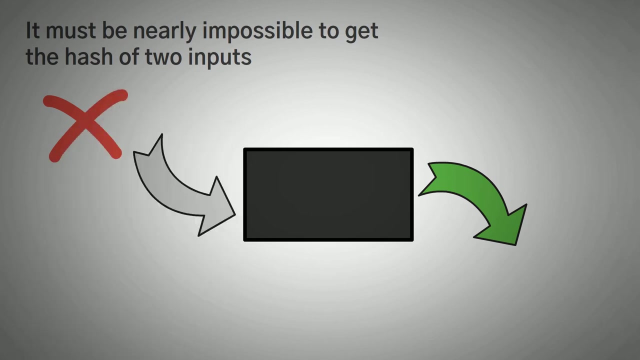 of the whole hashing algorithm, Number five. lastly, it must be nearly impossible to get the hash of two inputs equal to the same output. In fact, currently there are no known two inputs that generate the same output in SHA-256.. However, in MD5, which is a different hashing function, that 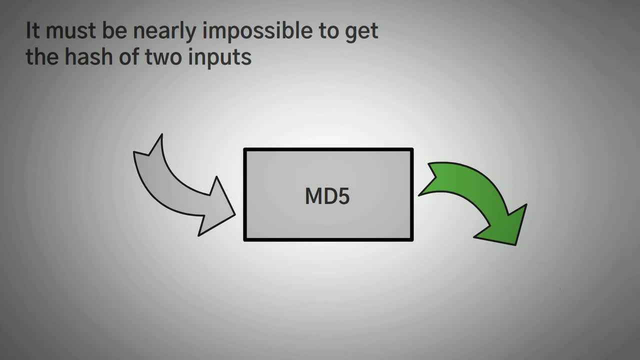 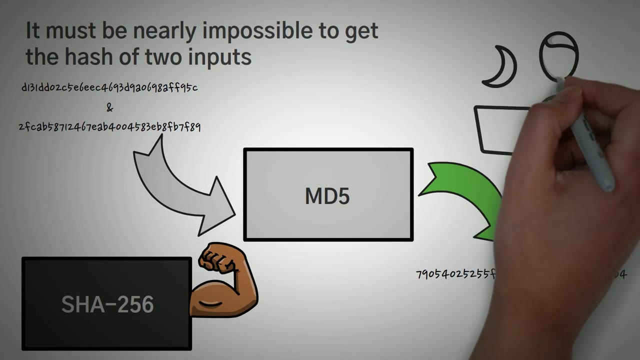 has a different magical black box and does different math, does have a few, For example, this input and this input. however, there aren't very many of these collisions found, And SHA-256 is much, much, much stronger than MD5. So people have actually been mining for years, while creating billions of 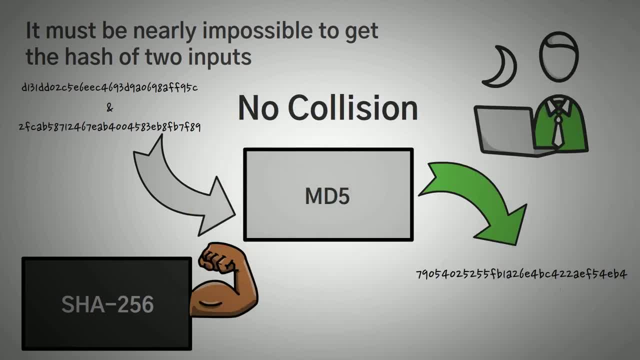 billions of SHA-256 hashes and no collision has been found. Maybe, if you're lucky, you'll find it yourself and you'll probably honestly win an award, But you just need to know two inputs. rarely, if not never, come up with the same hash. So, finally, what does all of this? a cryptographic 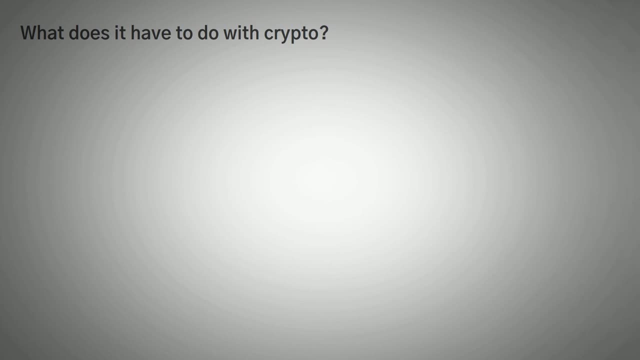 hashing function have to do with crypto. Well, it really has to do with something called proof of work, which is the exact method we use to actually mine Bitcoin. You can watch my proof of work video about it, but essentially here's. 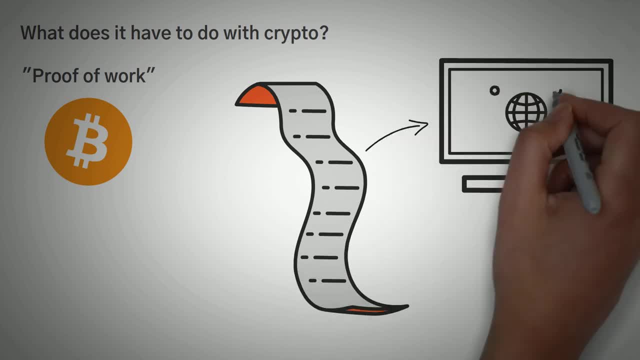 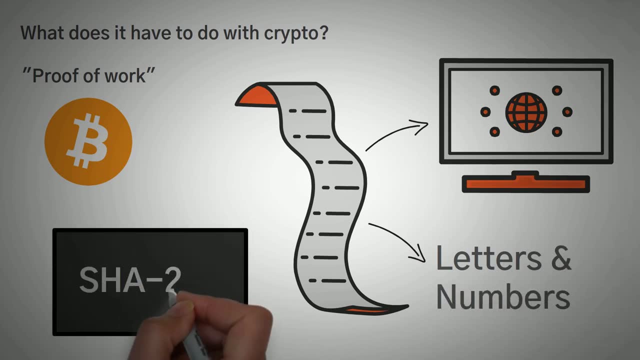 what we're doing. Number one: we're taking a list of all the transactions that people want added to the blockchain. Number two: we are then adding a random set of numbers and letters to that transaction list And finally, we are calculating the SHA-256 of that until we get an output that 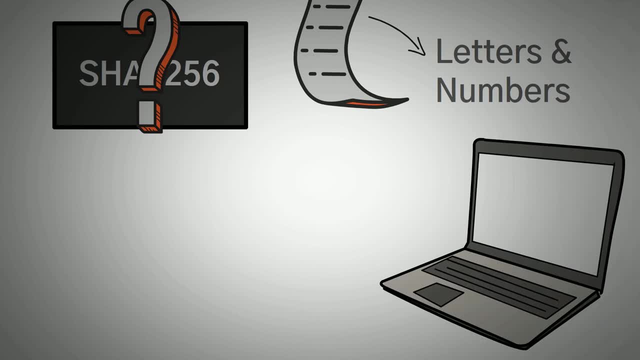 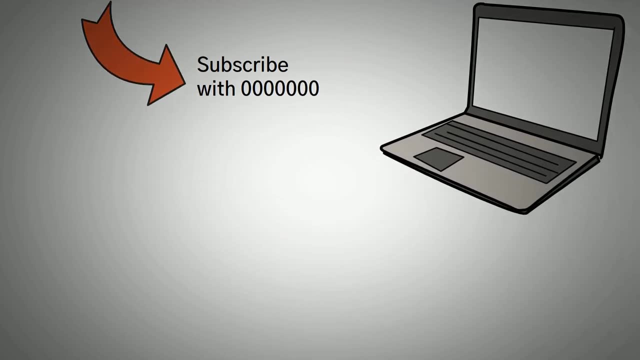 has a certain number of zeros. So in this case, because all I have right now is my personal computer, we're going to find out how to get subscribed to the blockchain And, finally, we're going to start with subscribe with seven zeros. Well, as we mentioned earlier, we can't predict. 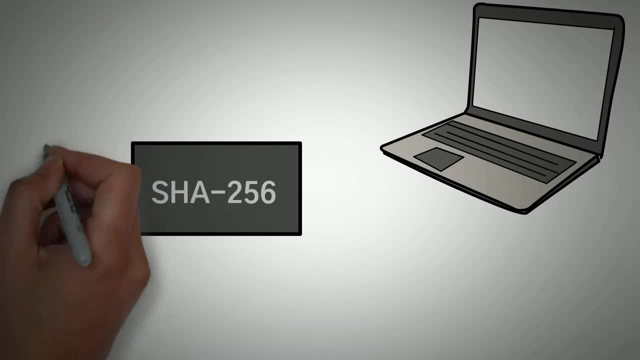 what we need to add to it, so we'll just have to guess and check. Let's start with one and then go up from there. So we start with subscribe one and this is what we get. It does not end with a. 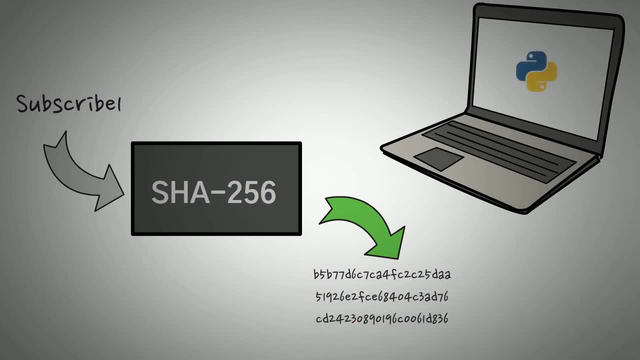 zero, it ends with a six. Then, using some simple Python code, we can keep adding a new number at the end until we get a zero at the end of the hash. For example, at subscribe nine, we get this, which has one zero. At subscribe 45, we get this, which is two zeros. On try number 2,864, we get 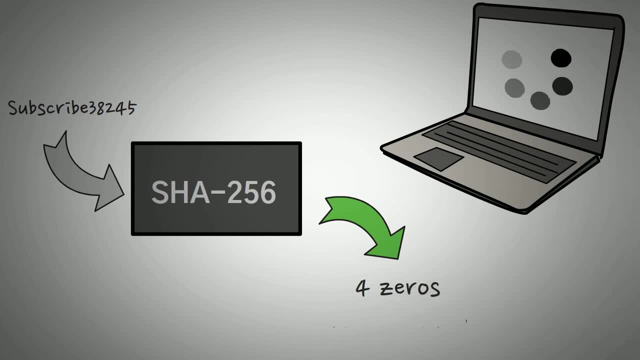 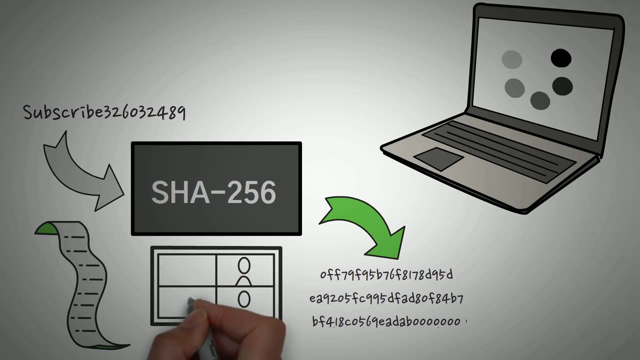 four zeros On try number 38,245,. we get four zeros, and so on and so on, Until subscribe 326,032,489,. we actually end up with seven zeros. Now, this is essentially what mining Bitcoin is, except, instead of subscribe, the data is literally a list of people exchanging Bitcoin. 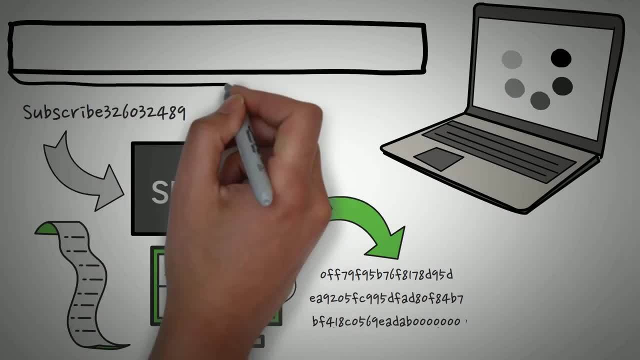 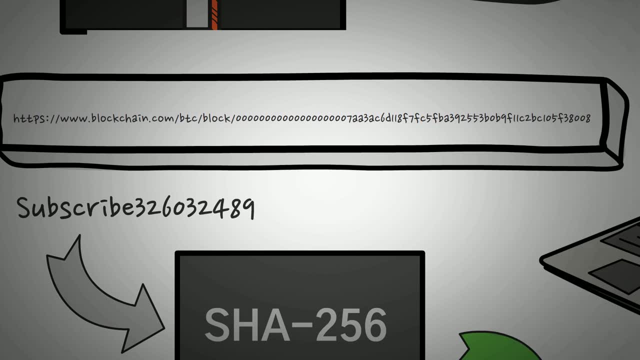 like John pays Bill five, Eric pays Robin eight, you pay me 20, and so on. And just to prove this, if you look at a recent Bitcoin block, you see that someone had to compute 19 zeros for the block to be valid, which my computer took 10 minutes to find. seven And, as you saw, 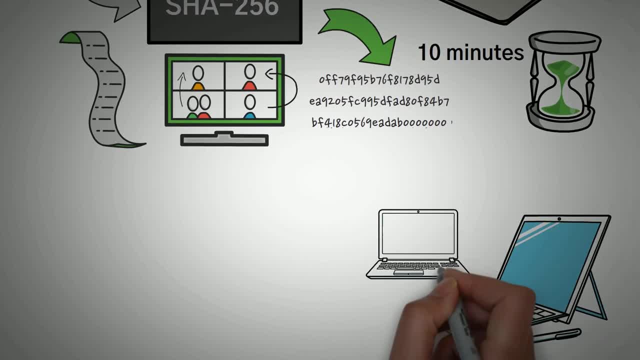 it exponentially took a lot more tries to get to the next zero. Now there are actually hundreds of thousands of computers around the world guessing all these random numbers and then once they find it- because we can pretty much make sure that they guessed and checked and didn't just